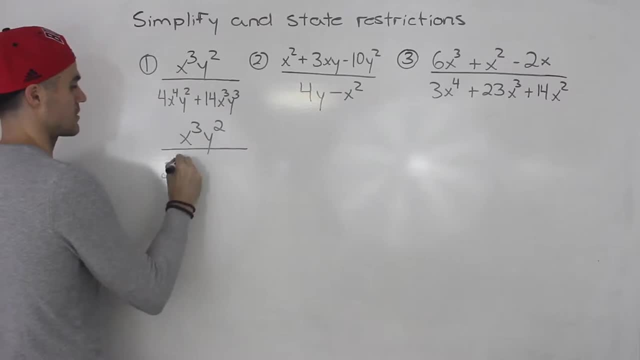 we got x to the 4, x to the 3, so we would take out an x to the 3.. then we got y2, y3, so we would take out a y2. so what would we be left with in the bracket? well, 4 x to the 4, y. 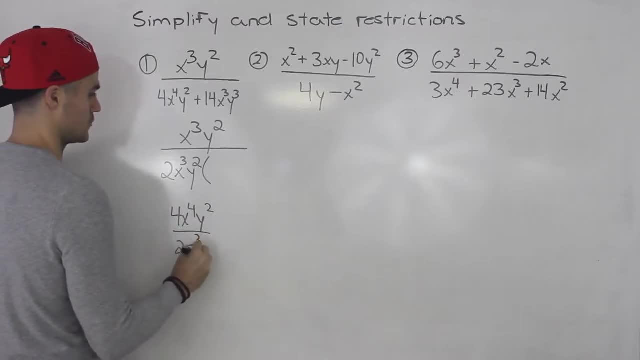 squared. divided by what we took out, 2 x cubed y squared, the y squares cancel out: 4 over 2 is just 2, and then x over 4 divided by x over 3 is just x. so we're left with 2x here and then um. 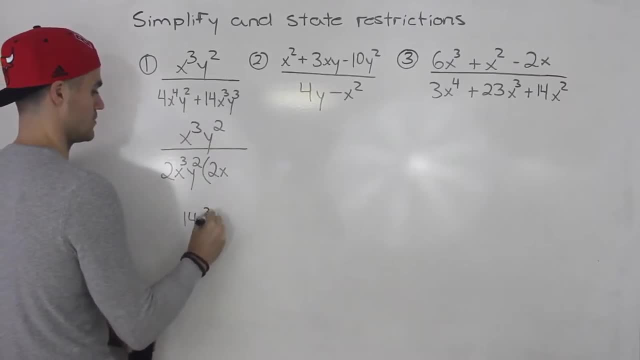 this one. we got 4x x cubed- y cubed over 2x cubed y squared. this, this cancel out. 14 over 2 is 7, y cubed over y squared is just y. so it ends up like that, right? so we factored next set. before we simplify, we 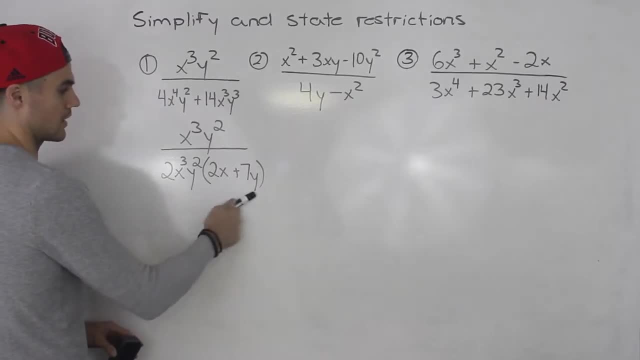 want to get the restrictions. so when can the denominator equal zero? basically, when x is zero. so that means x cannot equal zero, y cannot equal zero, right? the x and y are by themselves. and then also 2x plus 7y cannot equal zero. and now, at this point, what you want to do is you want to 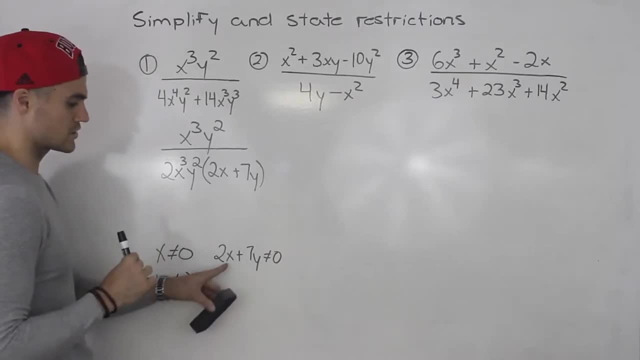 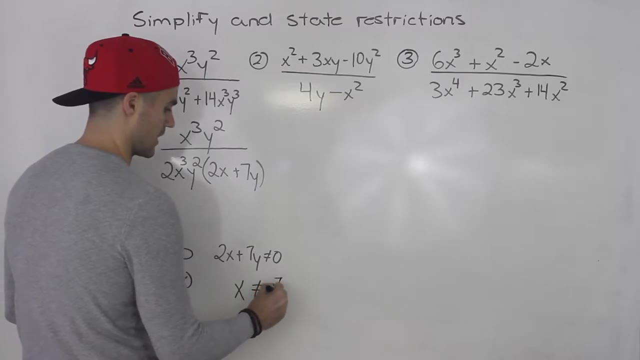 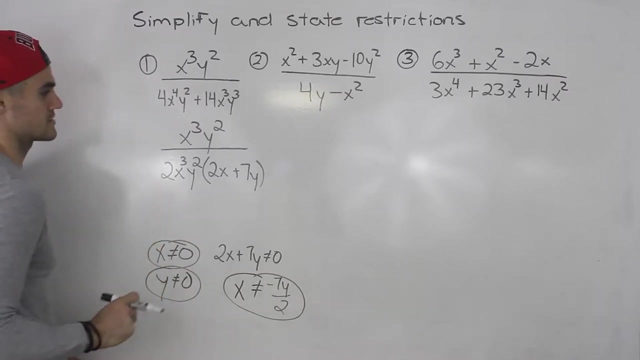 pick one of the variables to isolate for. personally, usually i pick the x, so if i isolate for x, i bring this over. we would have negative 7y over 2.. those are the three restrictions for this over here, and then, to simplify, we basically look: 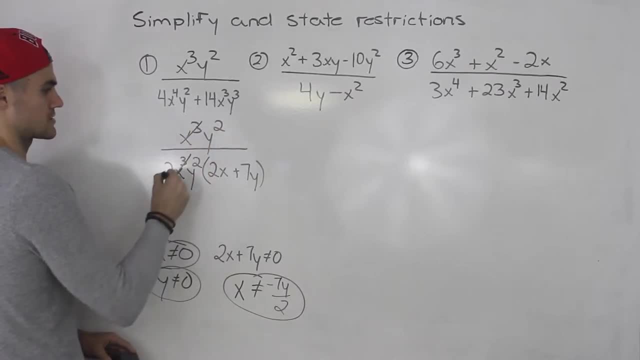 what can cancel on the numerator and the denominator: x cubed, x cubed, y squared, y squared and then nothing else. so we'd be left with one at the top and then two over here and then in brackets two x plus seven y. so that is what it simplifies to. these are the. 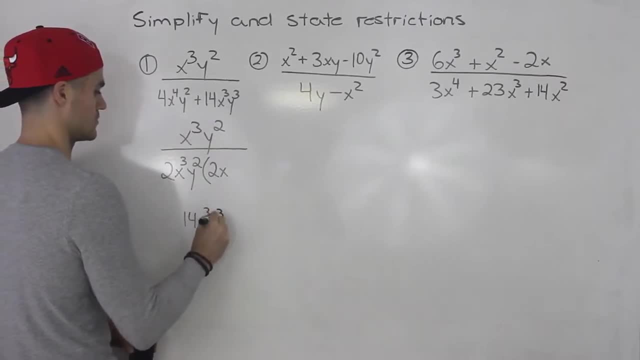 this one. we got 14 x cubed y cubed over 2 x cubed y squared. this, this cancel out. 14 over 2 is 7, y cubed over y squared is just y. so it ends up like that, right? so we factored next set. before we simplify, we 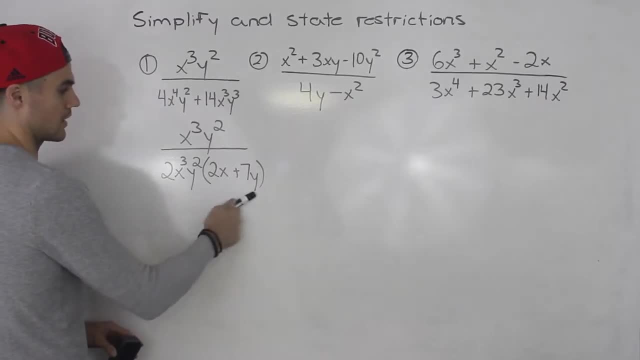 want to get the restrictions. so when can the denominator equal zero? basically, when x is zero. so that means x cannot equal zero, y cannot equal zero, right? the x and y are by themselves. and then also 2x plus 7y cannot equal zero. and now, at this point, what you want to do is you want to 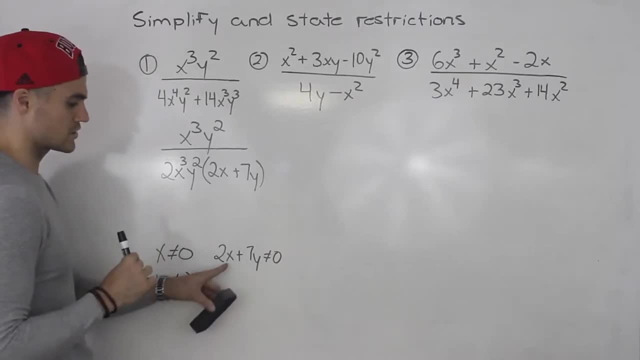 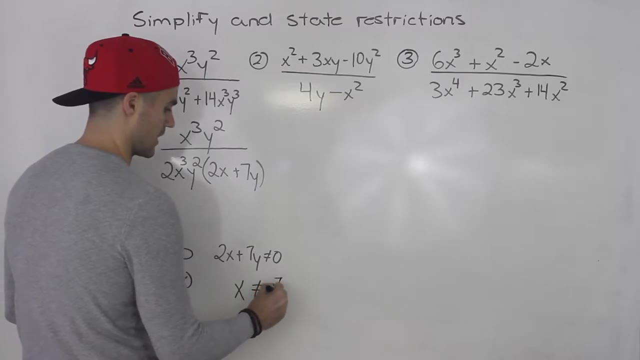 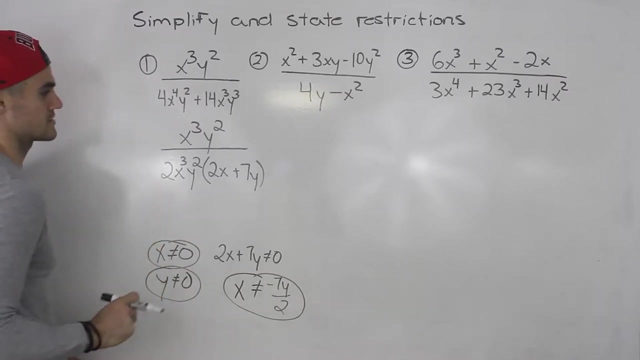 pick one of the variables to isolate for. personally, usually i pick the x, so if i isolate for x, i bring this over. we would have negative 7y over 2.. those are the three restrictions for this over here, and then, to simplify, we basically look: 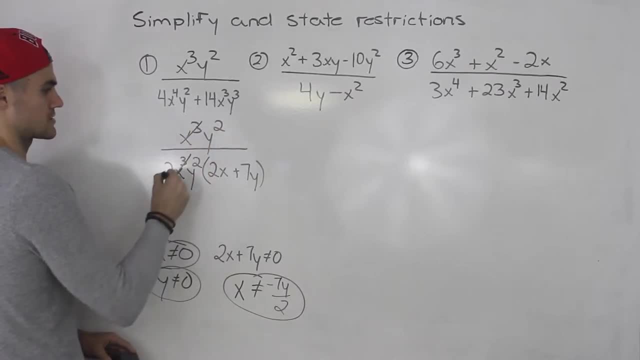 what can cancel on the numerator and the denominator: x cubed, x cubed, y squared, y squared and then nothing else. so we'd be left with one at the top and then two over here and then in brackets 2x plus 7y. so that is what it simplifies to. these are the. 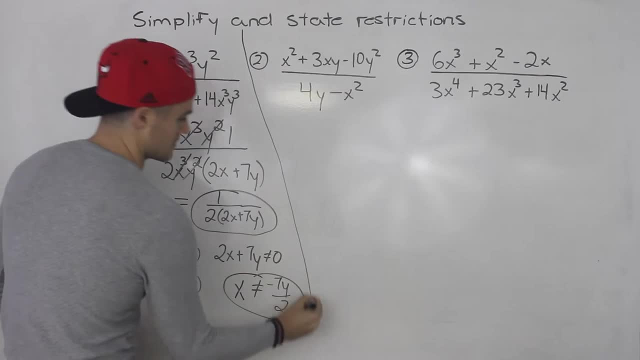 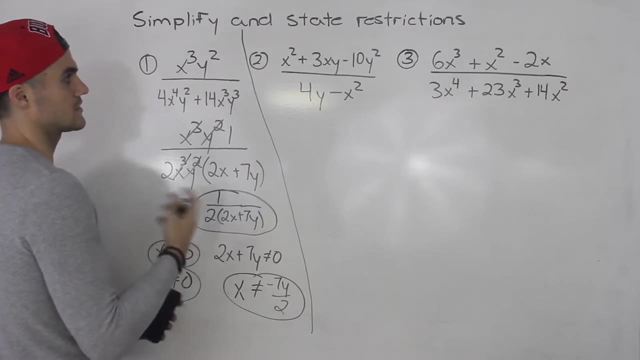 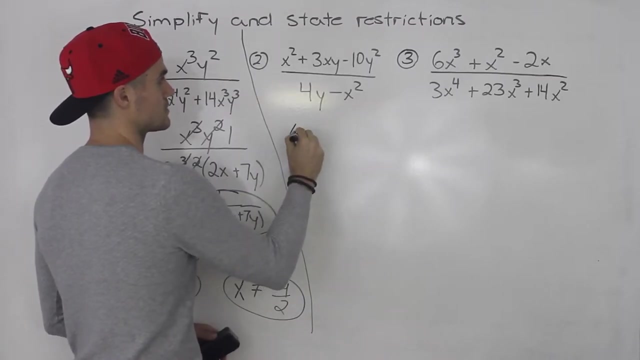 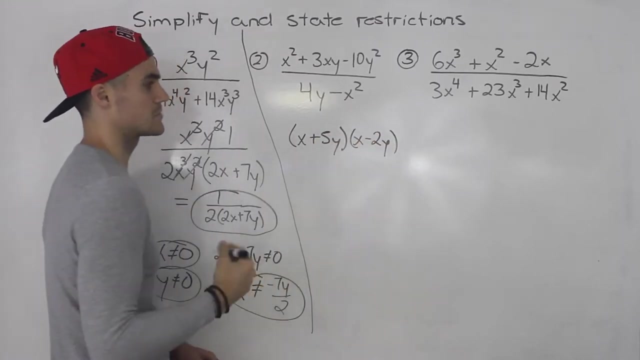 three restrictions. okay, moving on to number two, what you want to do, first step is you want to factor. now we've done tons of examples where we're factoring a quadratic with two variables in it. basically, this here would factor into x plus 5y and then x minus 2y once you do the decomposition. 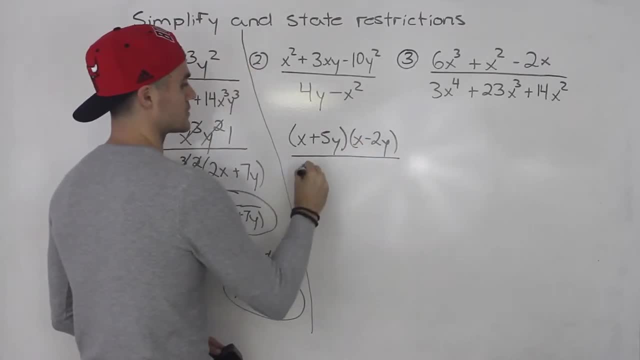 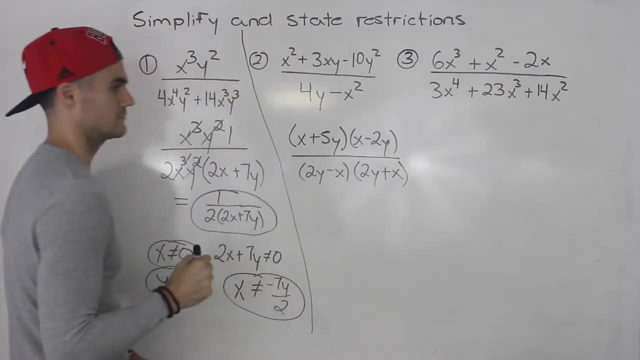 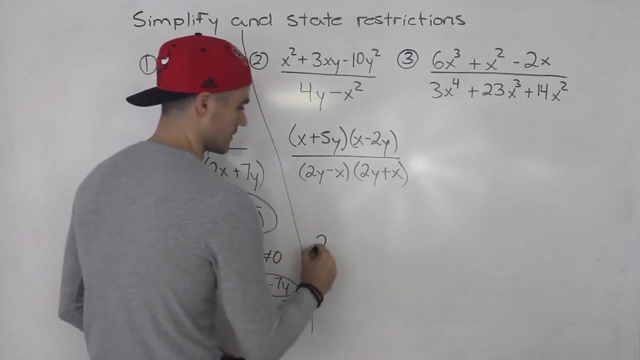 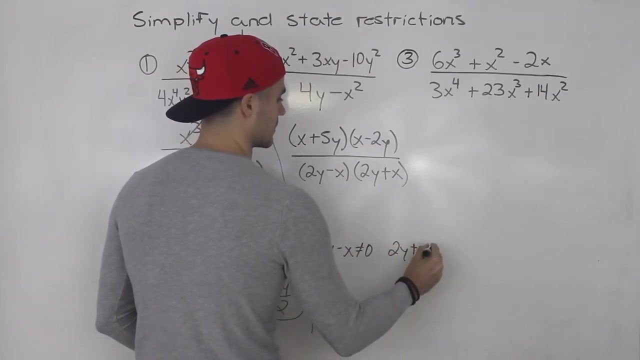 and then the denominator that would factor into two, and then the denominator that would factor into 2y minus x, and then 2y plus x, like that, and then from here you want to state the restriction. so basically 2y minus x cannot equal 0 and 2y plus x cannot equal 0, and then in my opinion it's easiest to: 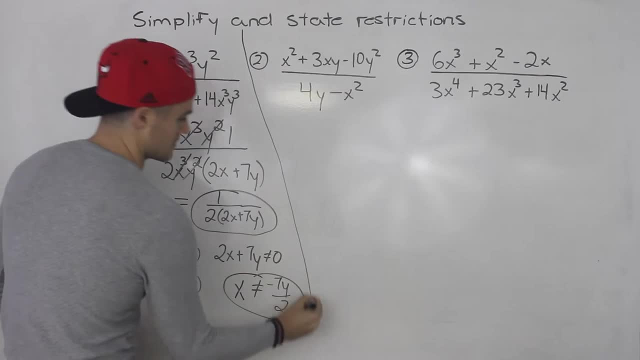 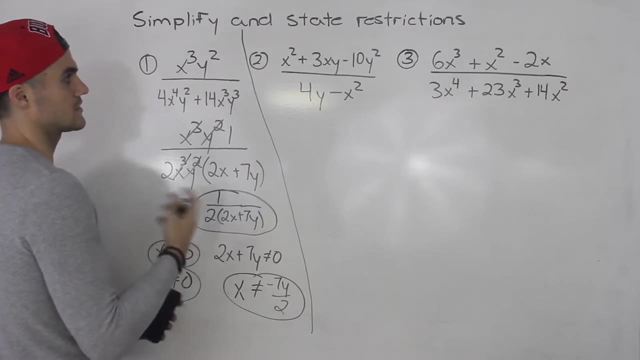 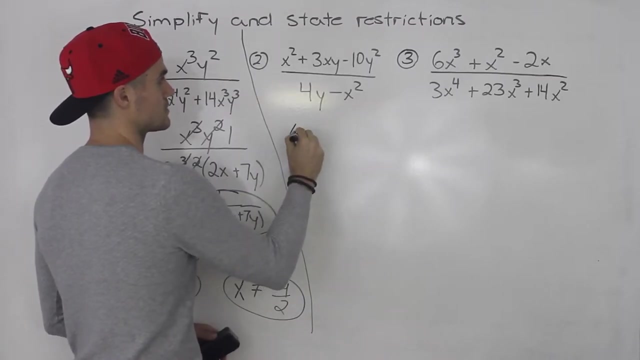 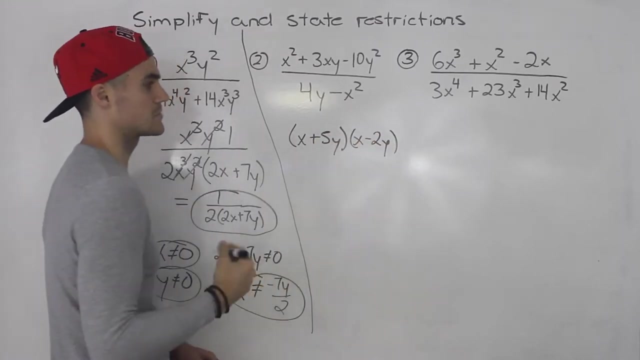 restrictions. okay, moving on to number two, what you want to do first step is you want to factor. now we've done tons of examples where we're factoring a quadratic with two variables in it. basically, this here would factor into x plus 5y and then x minus 2y once you do the decomposition. 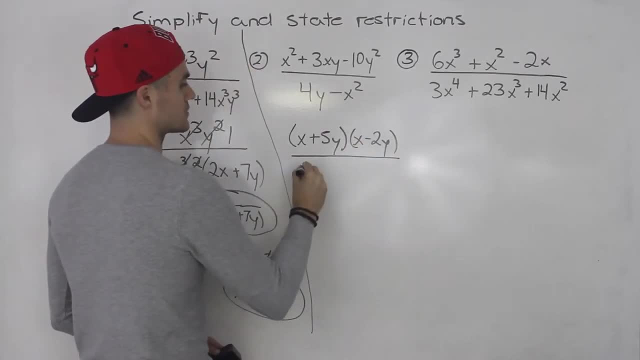 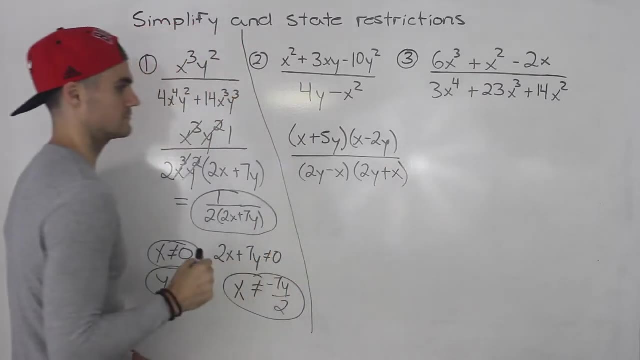 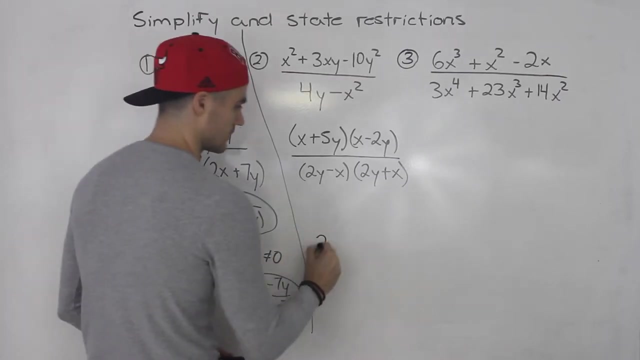 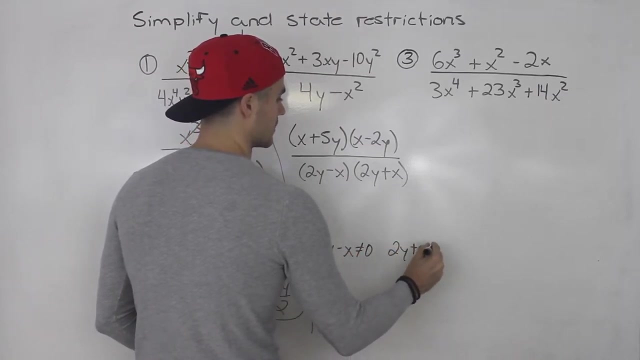 and then the denominator that would factor into two, and then the denominator that would factor into 2y minus x, and then 2y plus x, like that, and then from here you want to state the restriction. so basically 2y minus x cannot equal zero, and 2y plus x cannot equal zero, and then in my opinion it's easiest to isolate for the x's. so 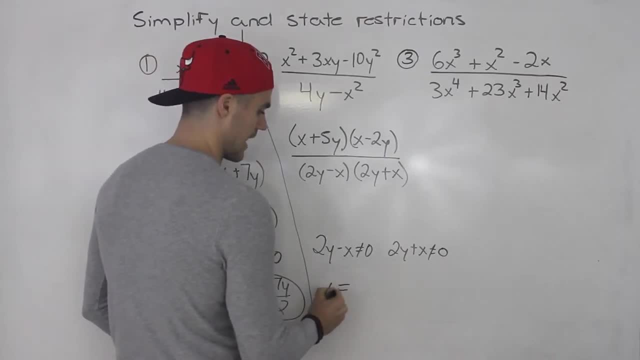 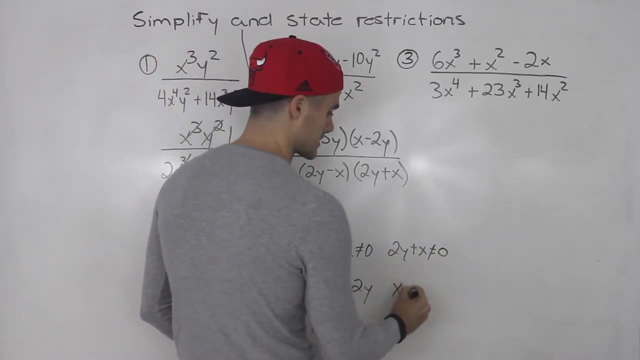 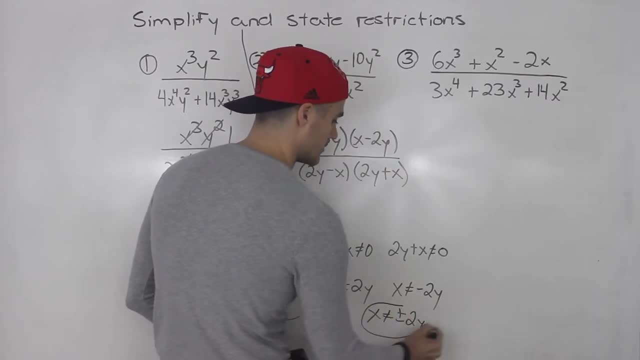 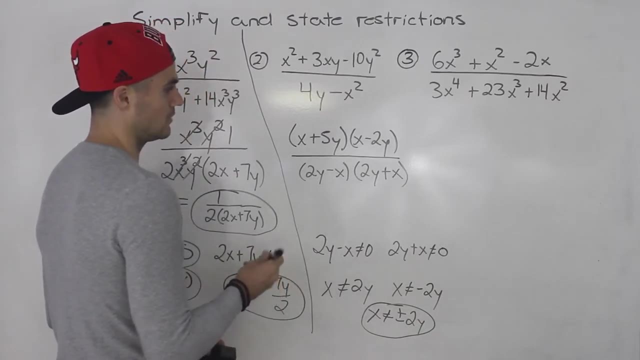 2y. that is the restriction. then from here, is there anything that could cancel out? well, notice that x minus 2y, 2y minus x. they are fairly similar, but not quite yet. but we can make them the same, so we can make them the same. so we can make them the same, so we can make them the same. 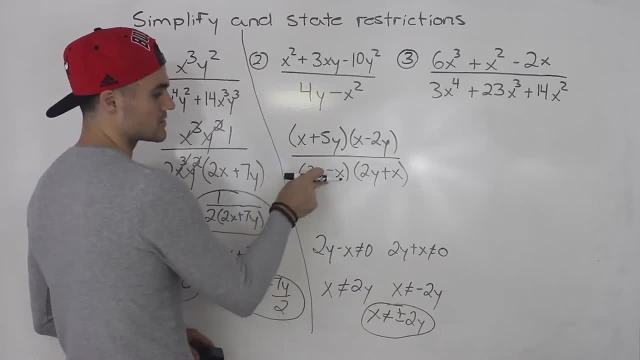 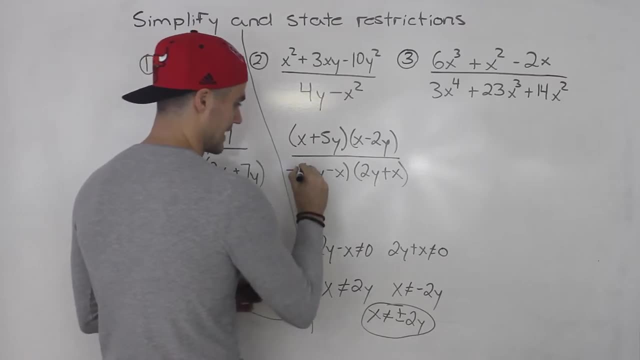 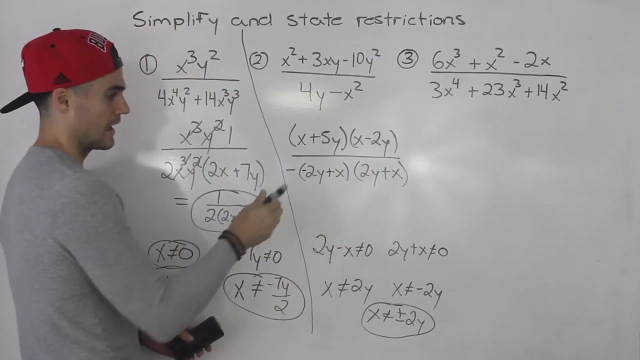 if we factor out a negative from either bracket. so i'm going to factor out a negative from this bracket. if i take out a negative from this bracket, i would be left with negative 2y plus x, like that. basically all the signs change and then negative 2y plus x. that's the same. 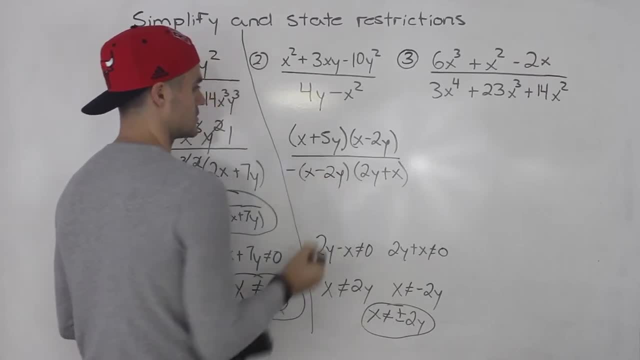 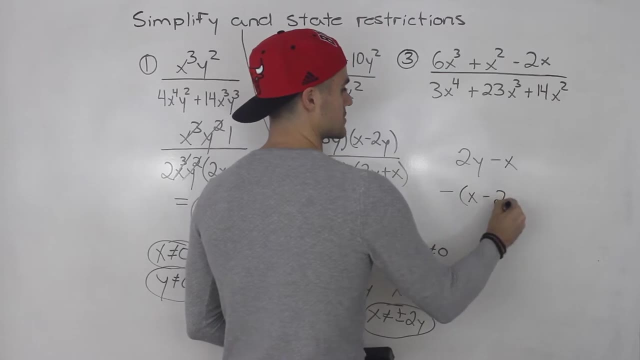 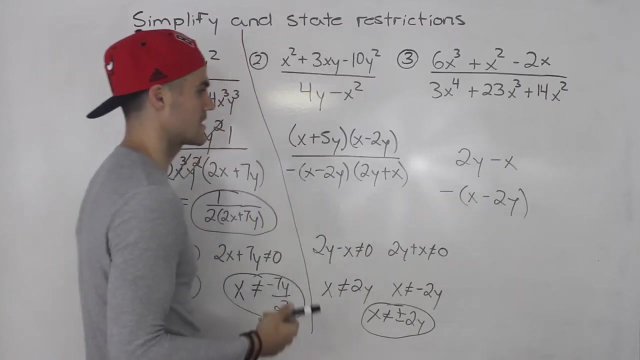 as x minus 2y, right. so basically 2y minus x is the same x as negative x minus 2y, Right. if we bring that negative back in negative, x plus 2y same as 2y minus x. And the reason why we want to do that? because now these can cancel out. So what does? 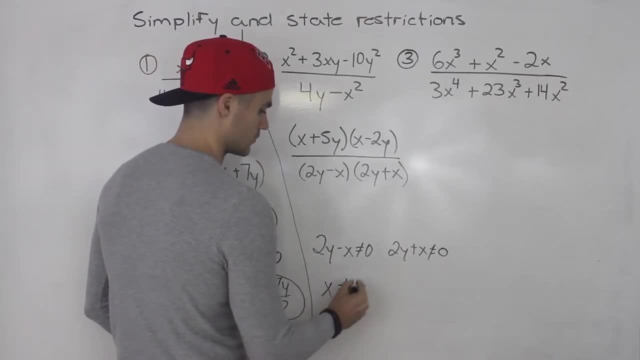 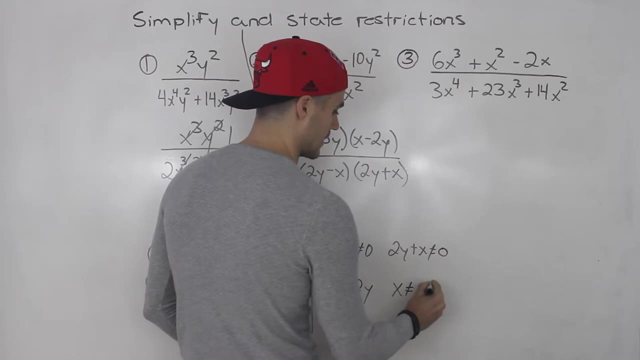 isolate for the x's. so the negative x we bring over. so the x's cannot equal 2y, and then x here is positive, so let's bring the 2y over and then over. here x cannot equal negative 2y and then, if you want to put these in one, basically x cannot equal. 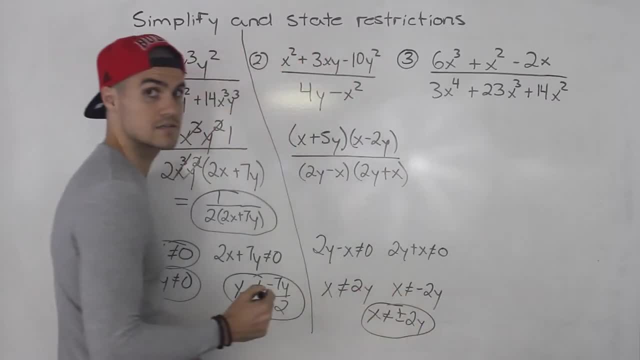 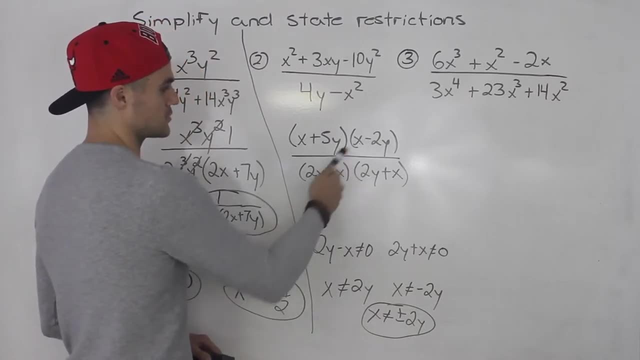 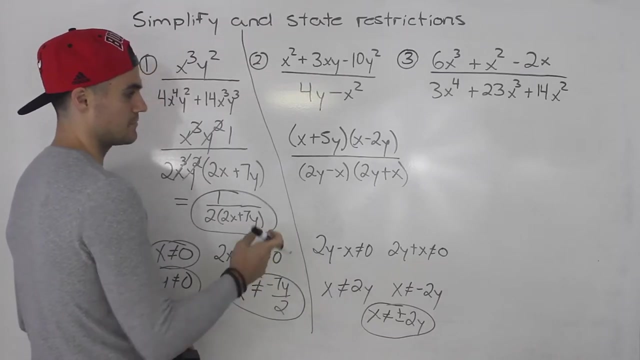 plus or minus 2y. that is the restriction. then from here, is there anything that could cancel out? well, notice that x minus 2y, 2y minus x, they are fairly similar, but not quite yet. so what we're going to do is we're going to do the same if we factor out a negative from either. 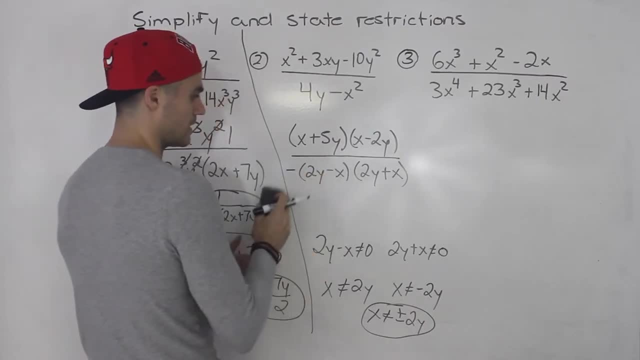 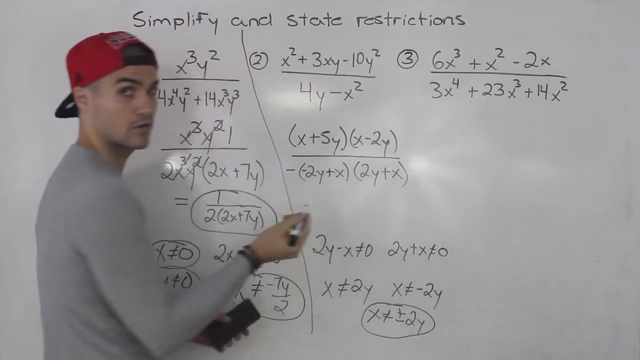 bracket. so i'm going to factor out a negative from this bracket. if i take out a negative from this bracket, i would be left with negative 2y plus x, like that. basically all the signs change and then negative 2y plus x, that's the same. 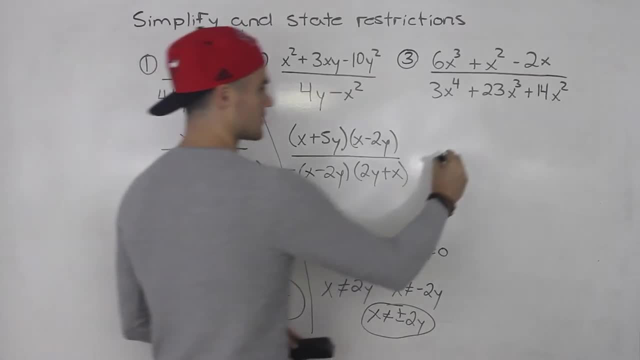 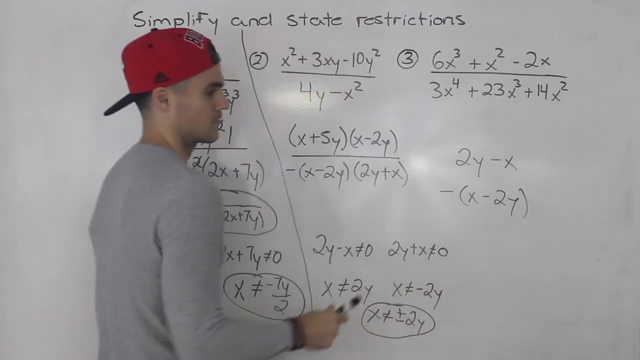 as x minus 2y, right? so basically, 2y minus x is the same as negative, 2y, negative, x minus 2y, right? if we bring that negative back in, negative, x plus 2y same as 2y minus x. and the reason why we want to do that: 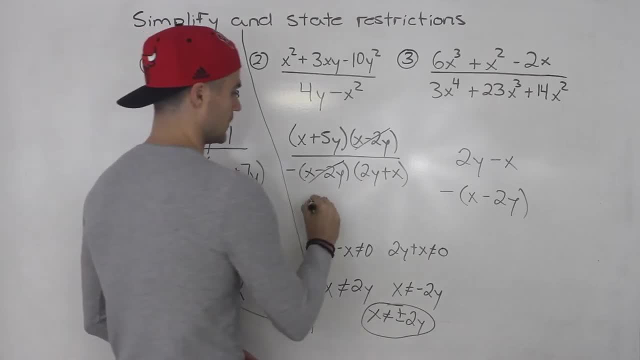 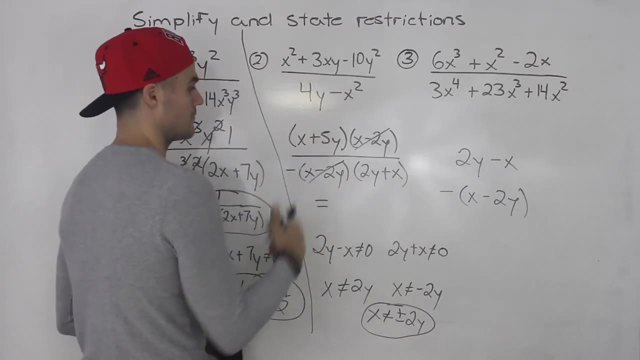 because now these can cancel out. so what does this simplify? to well, this negative we could keep in the denominator. i usually like to just bring up any negatives to the numerator, if possible. so bringing that up there, it's like that. and then 2y plus x. 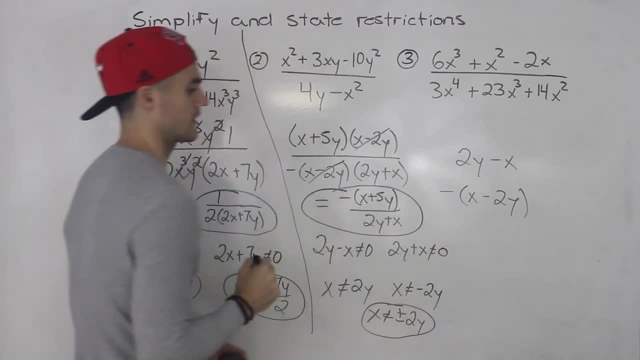 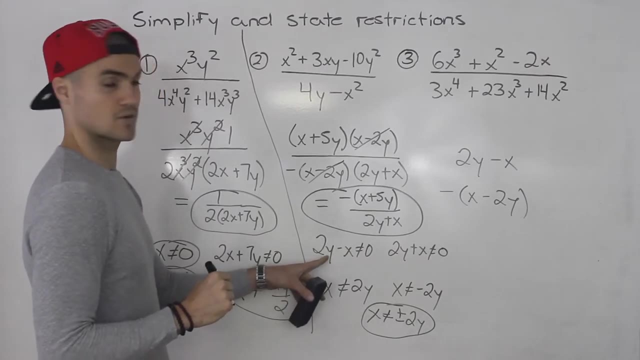 is left on the bottom, so that there is the final answer. that's what it simplifies, to that there is the restriction also here. note that you could have also isolated for the y in both of these, and if you do that, basically here y would. uh, y cannot equal positive x over two. here would: 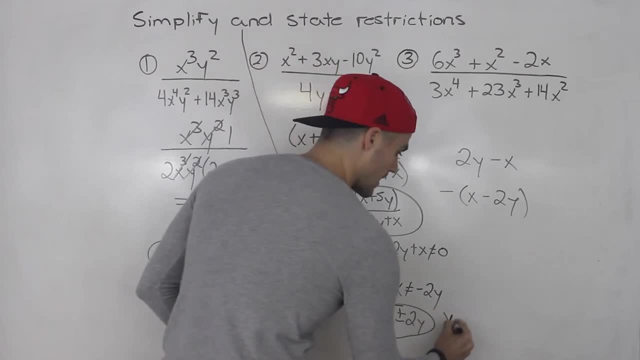 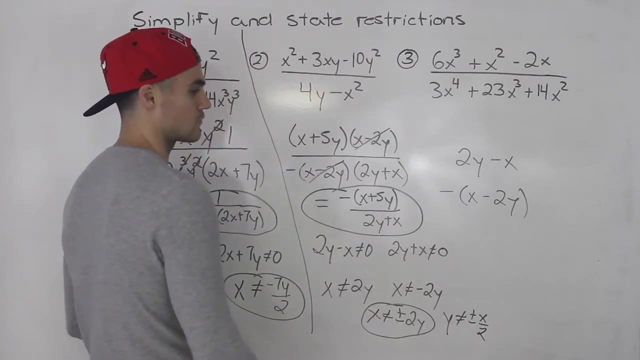 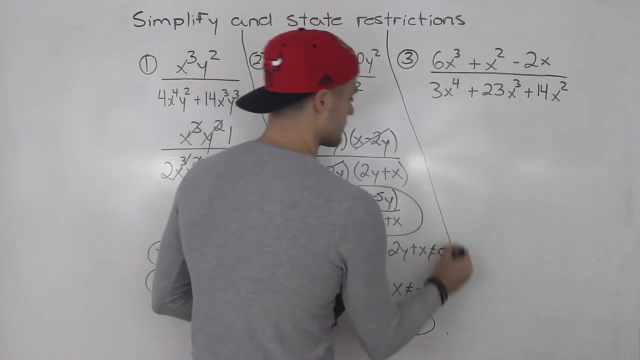 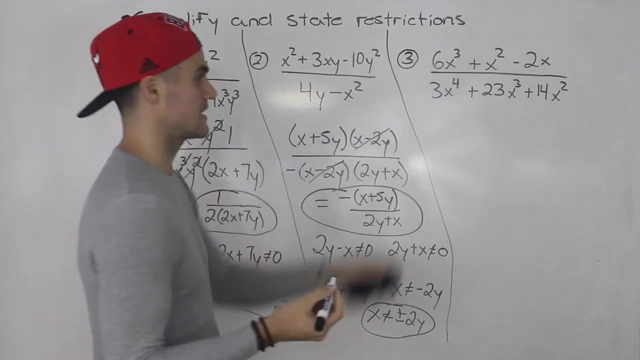 be negative x over two. so the other restriction is y cannot equal plus or minus x over two. so that works as well. but i isolated for the x. okay, so that's number two. and then finally number three: um, we got a factor. so notice from the numerator, we could take out an x first. so if we take out an x, we'll be left with six x squared. 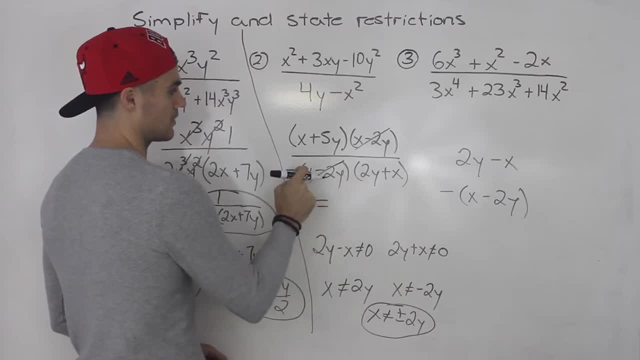 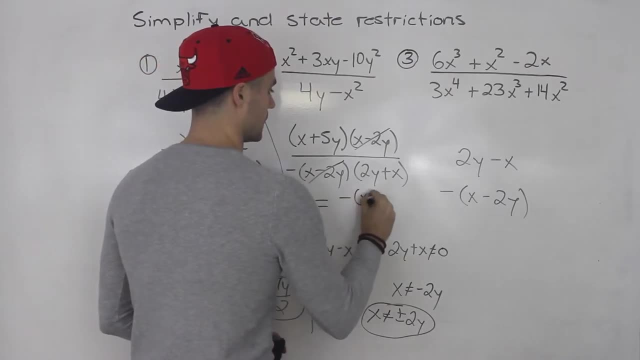 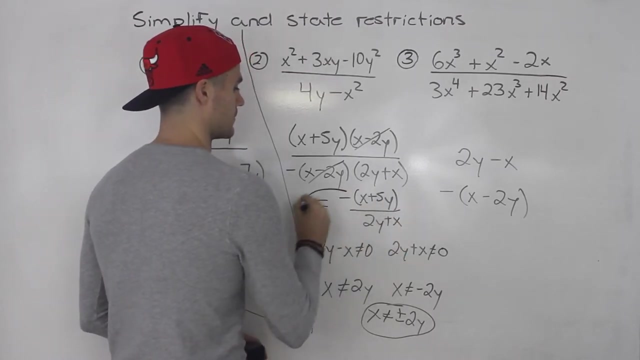 this simplify to. Well, this negative we could keep in the denominator. I usually like to just bring up any negatives to the numerator, if possible. So bringing that up there, it's like that, and then 2y plus x is left on the bottom, So that there is the final answer. That's what it simplifies to. 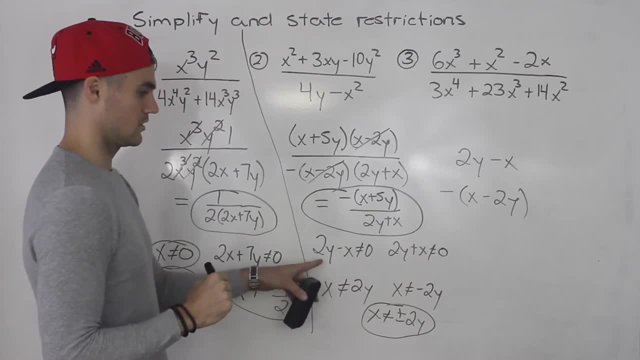 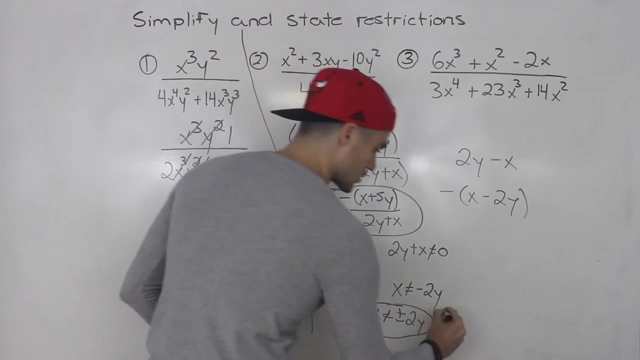 that there is the restriction Also here. note that you could have also isolated for the y in both of these, And if you do that, basically here y cannot equal positive x over 2, here would be negative x over 2.. So the other restriction is: y cannot equal plus or minus x. 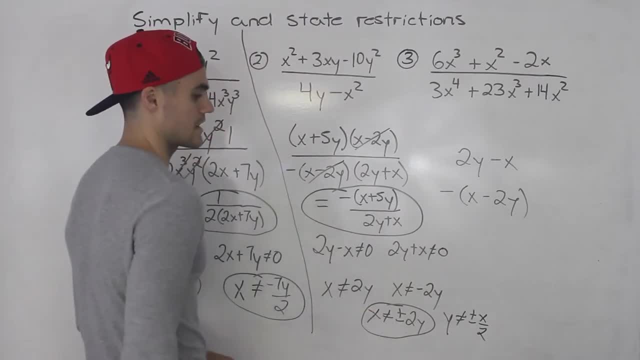 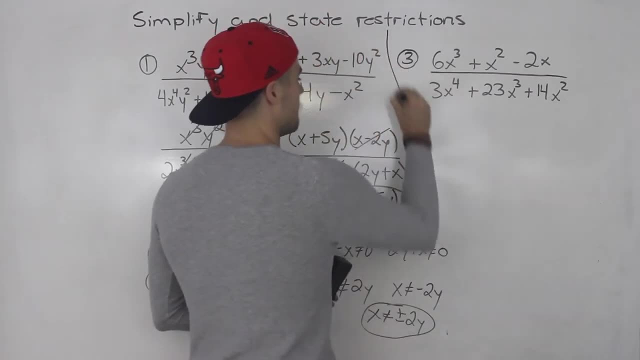 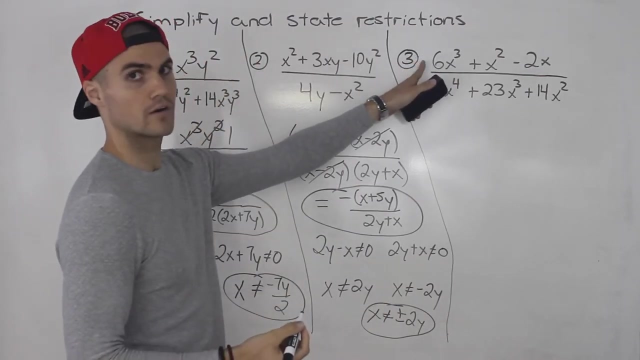 over 2.. So that works as well. but I isolate it for the x. Okay, so that's number 2.. And then finally number 3, we got a factor. So notice, from the numerator we could take out an x first. So if we take out, 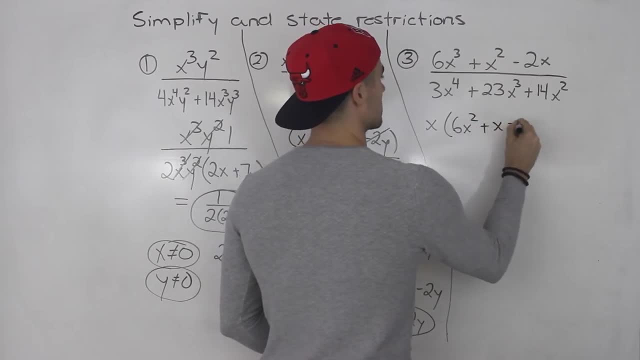 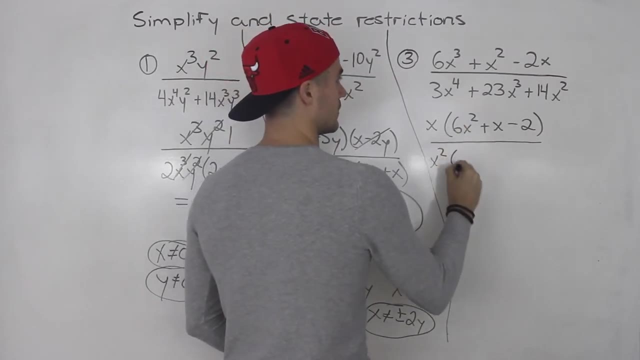 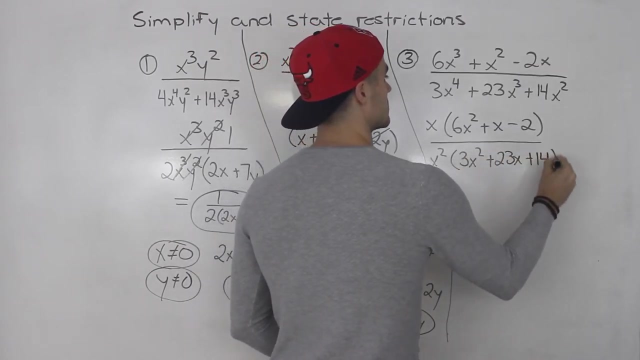 an x, we'd be left with 6x squared plus x minus 2.. And then over here from the denominator, we could get an x squared And we'd have 3x squared plus 23x plus 14.. And then we have to factor these two. 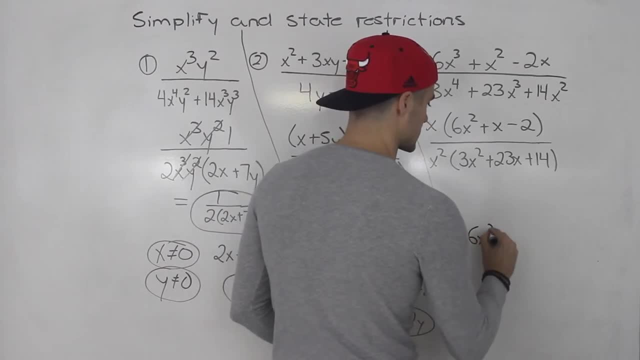 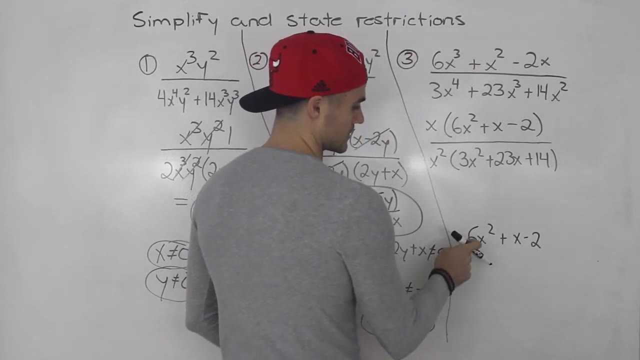 quadratics. So I'm actually going to do it on the side here. So 6x squared plus x minus 2. That would be what? So two numbers that multiply negative 12 add up to 1. That would be 4x. 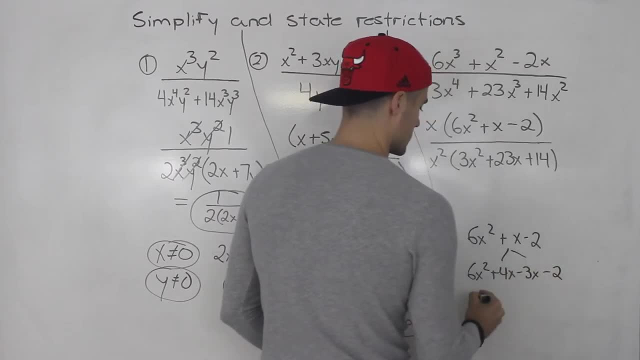 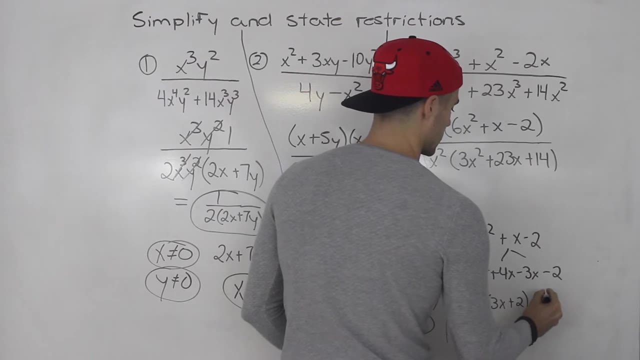 And minus 3x, So we could take out a 2x from both of these. So we'd be left with 3x plus 2.. Then we could take out a negative 1. And we'd be left with 3x plus 2.. And then these you could take. 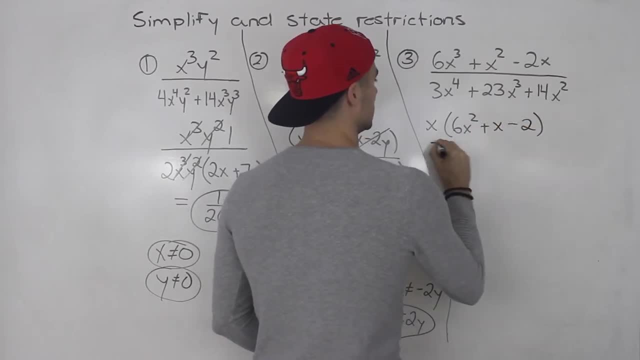 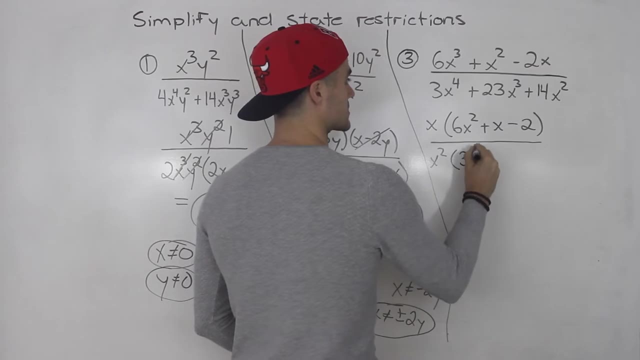 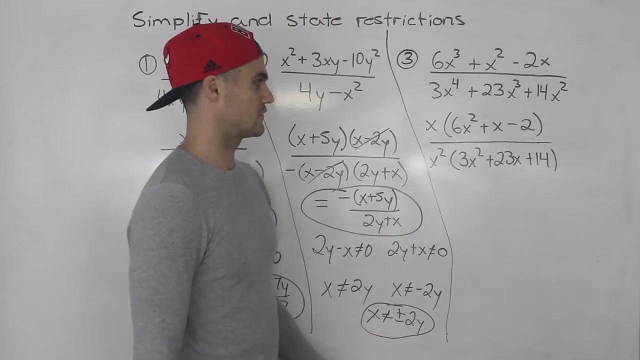 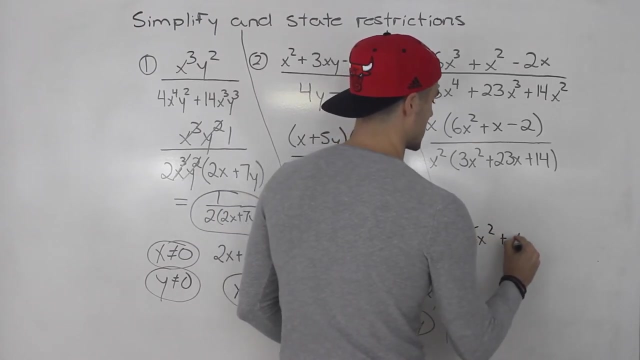 plus x minus two, and then over here from the denominator we could take out an x squared plus woo and we'd have 4x squared, and we'd have 4x squared plus 23 x plus 14.. and then we have to factor these two quadratics, so i'm actually gonna do it on the side here, so 6x squared. 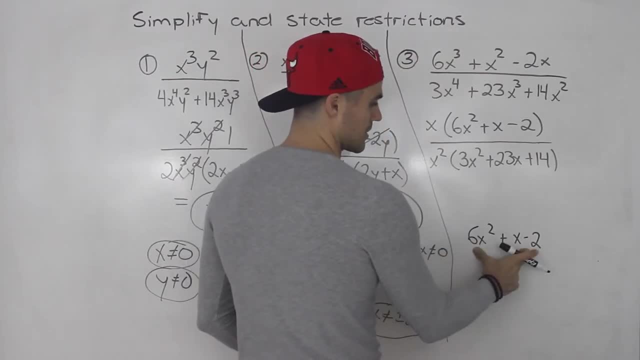 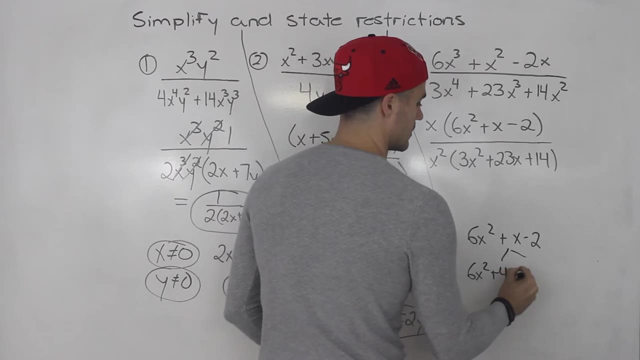 plus x minus 2, that would be what? so two numbers that multiply negative 12 out up to one. that would be um 4x and minus 2, 3x. So we could take out a 2x from both of these. so we'll be left with 3x plus 2. 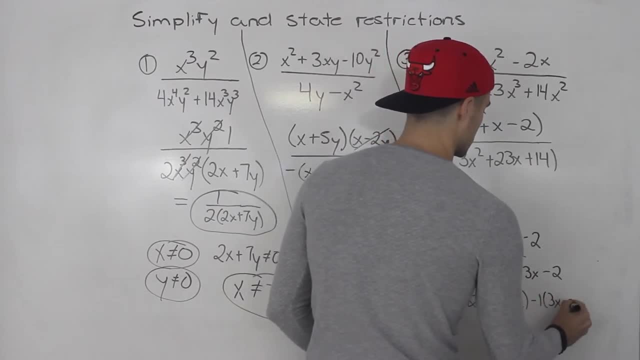 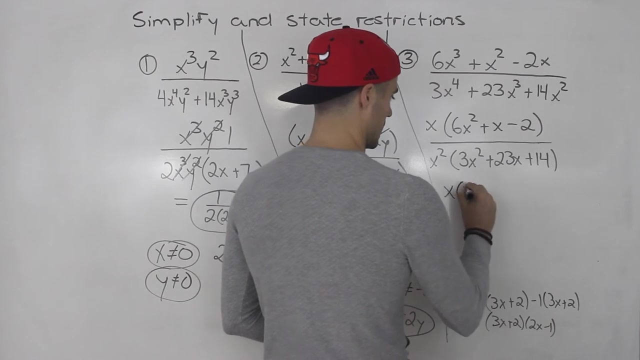 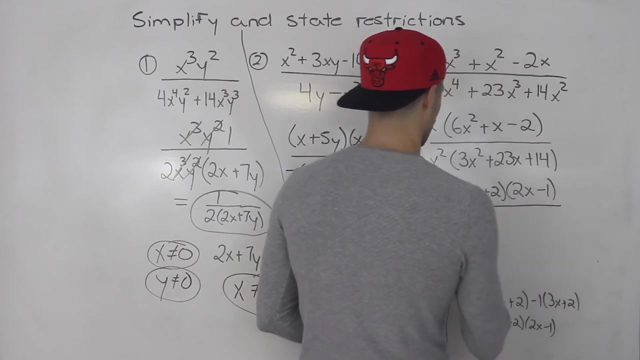 then we could take out a negative 1 and we'll be left with 3x plus 2.. And then these: you could take out a 3x plus 2, left with 2x minus 1.. Okay, so the numerator factors into 3x plus 2 times 2x minus 1.. Denominator: we got x squared. 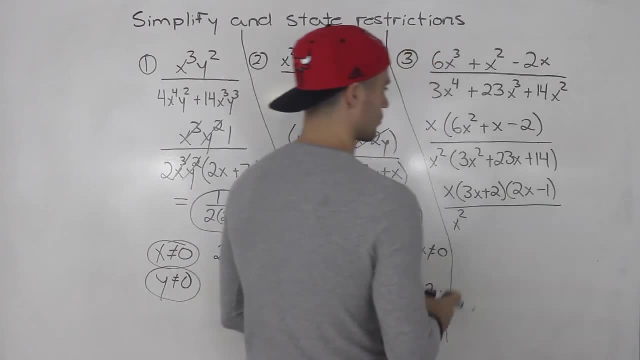 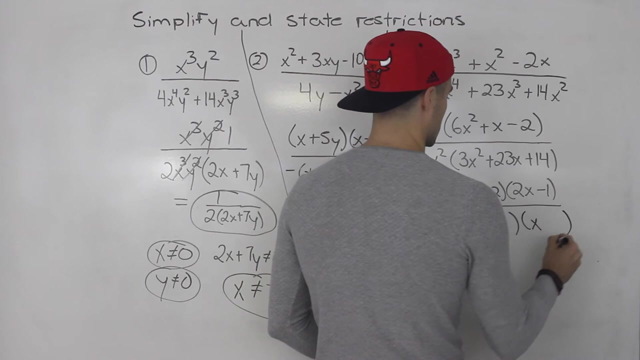 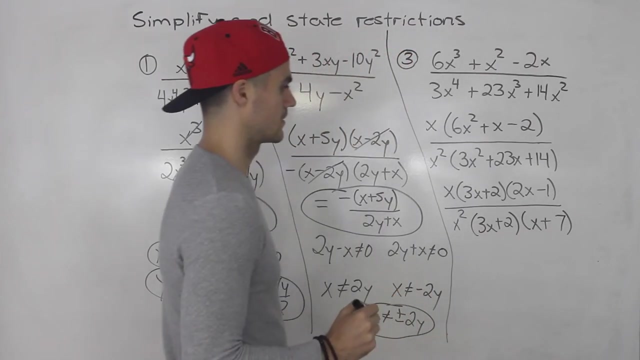 here at the bottom. and then what would 3x squared plus 23x plus 14 factor into? I think what it would be is it would be 3x there and then x over here. I'm pretty sure one of will be 3x plus 2. This would be x plus 7.. Alright, so that works. So if you do, 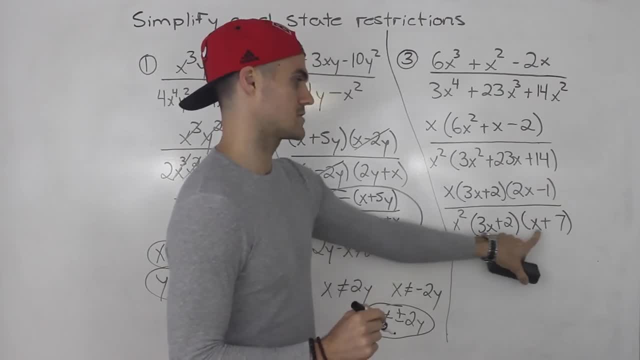 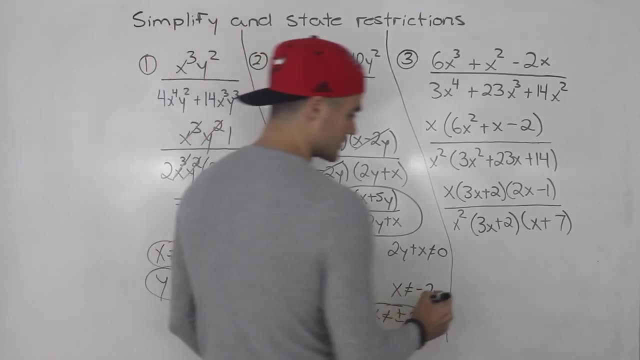 decomposition on this quadratic, you would end up with 3x plus 2, x plus 7.. And then from here, before you simplify, you want to get the restriction. So notice here: x cannot equal 0. That's one of the restrictions Here. if we let this whole, 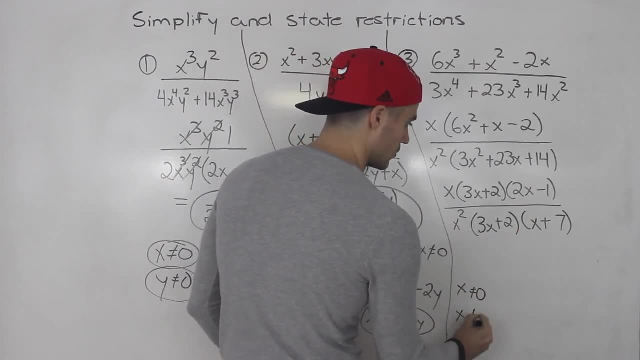 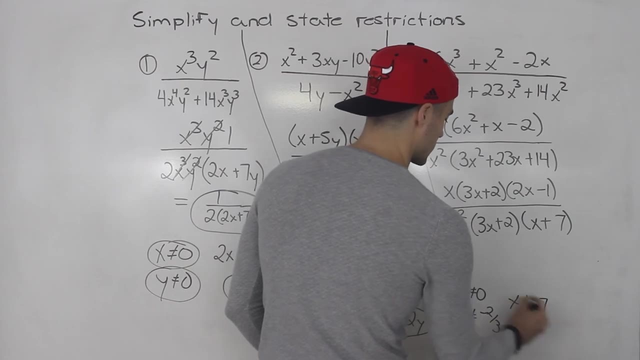 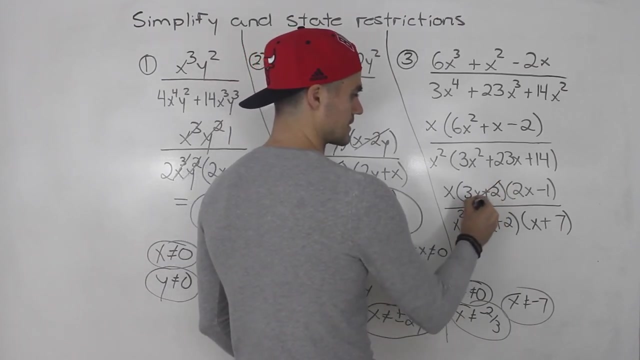 expression not equal 0. it means x cannot equal negative 2 over 3.. Then here, x cannot equal negative 7.. So these are the three restrictions, And then we could simplify. Notice that this and this cancel out, And then we have 1x at the. 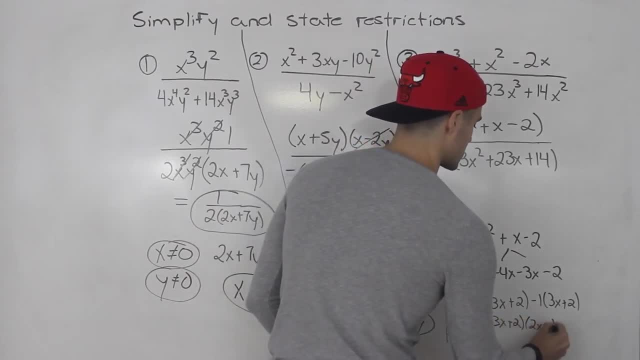 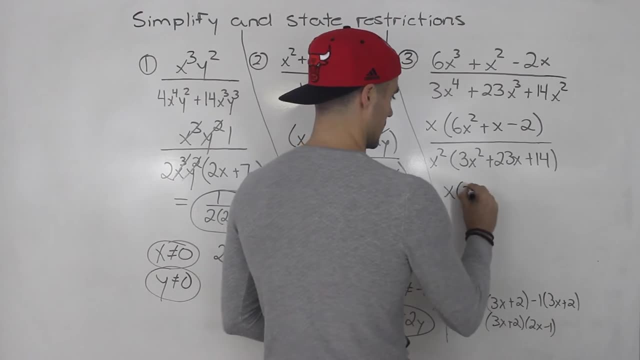 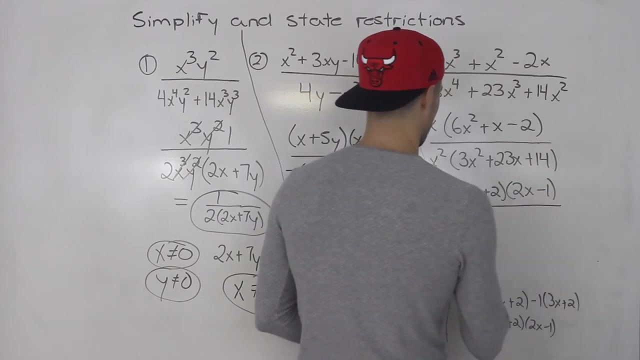 out a 3x plus 2, left with 2x minus 1.. Okay, so the numerator factors into 3x plus 2.. Times: 2x minus 1.. Denominator: we got x squared here at the bottom, And then what would 3x squared? 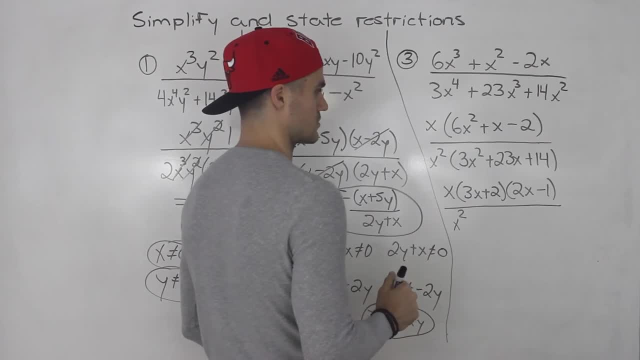 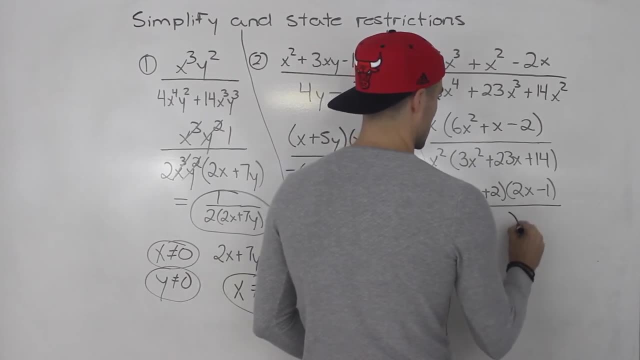 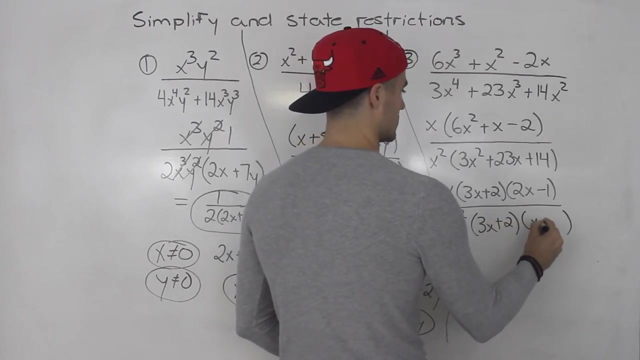 plus 23x plus 14. factor into, I think what it would be is it would be 3x there and then x over here, And I'm pretty sure one of them will be 3x plus 2. This would be x plus 7.. 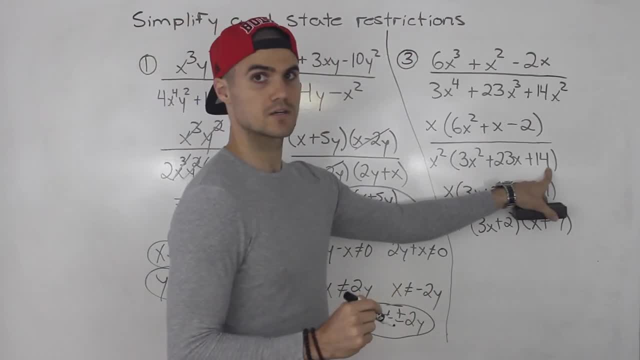 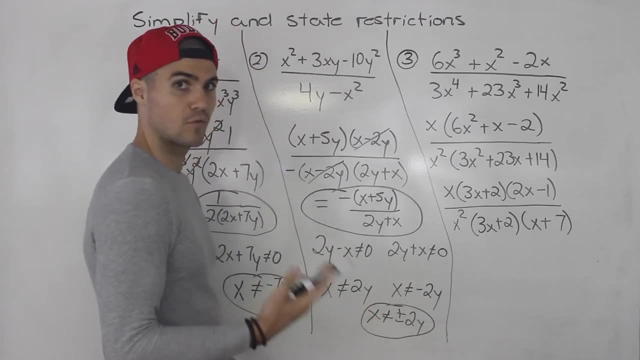 All right, so that works. So if you do decomposition on this quadratic, you would end up with 3x plus 2x plus 7.. And then from here, before you simplify, you want to get the restriction, So notice here. 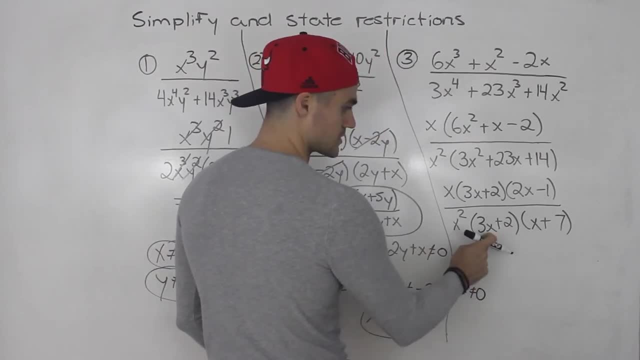 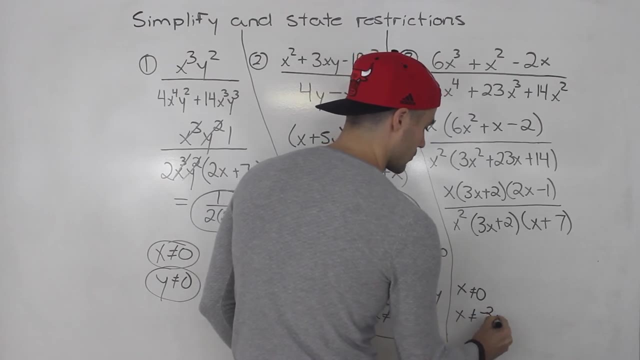 x cannot equal 0. That's one of the restrictions Here. if we let this whole expression not equal 0, it means x cannot equal negative 2 over 3.. And here x cannot equal negative 7.. So these are the three restrictions And then we could simplify. Notice that this and 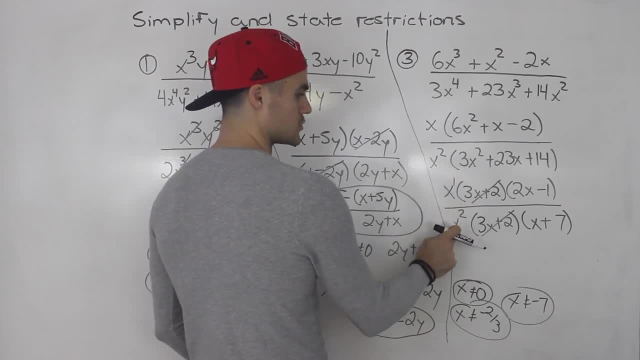 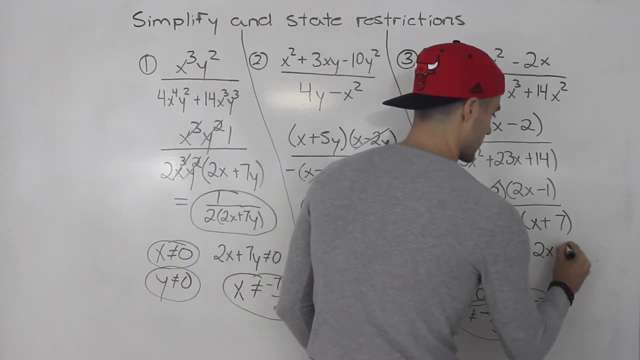 this cancel out. and then we have 1x at the top, 2x is at the bottom. So that means we're left with 1x at the bottom. So this simplifies to 2x minus 1.. That's the expression. 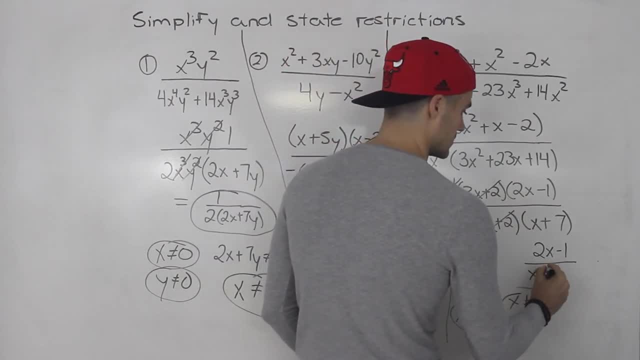 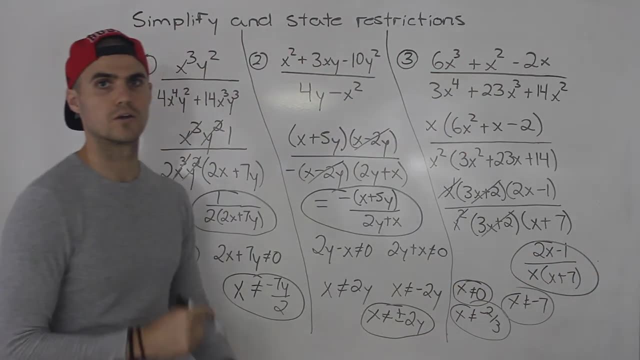 left in the numerator and then we got an expression x in the denominator and an x plus 7. So that's what it simplifies to Simplifies two. and those are the three restrictions. 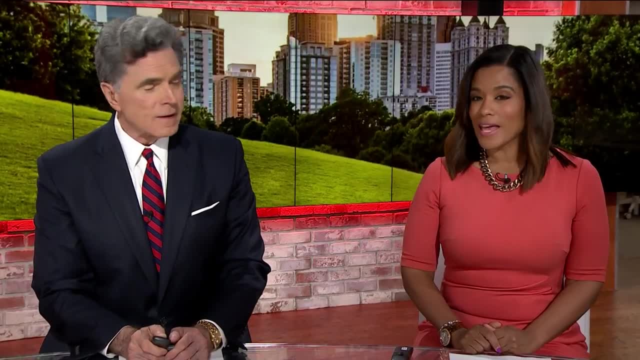 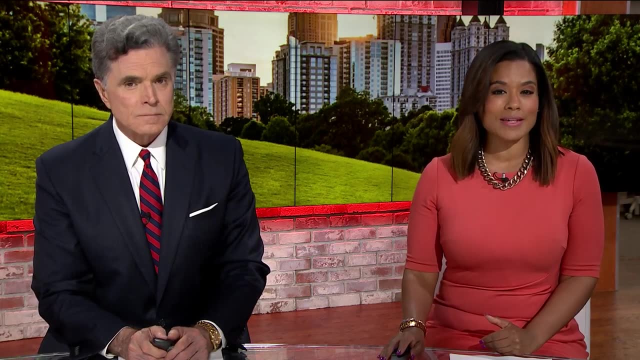 Now early voting for Georgia's primary election is underway And as we track the races, an 11 Alive viewer wanted more details about some of the non-candidate questions you could see on the ballot. Liza Lucas has your fast facts. Georgia voters have decisions to make and before heading to the polls, 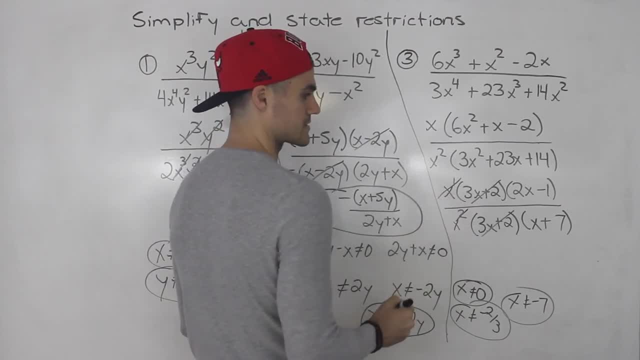 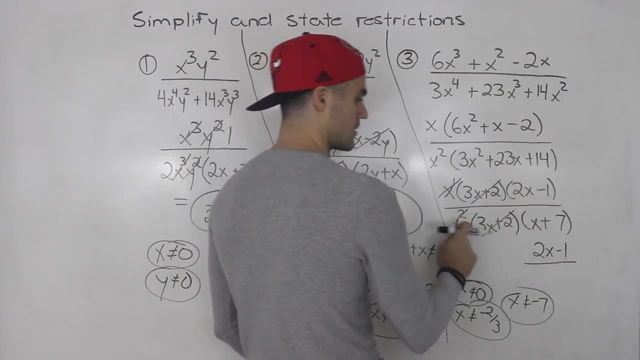 top 2x is at the bottom. So that means we're left with 1x at the bottom. So this simplifies to 2x minus 1.. Now the expression left in the numerator. and then we got an expression x in the.